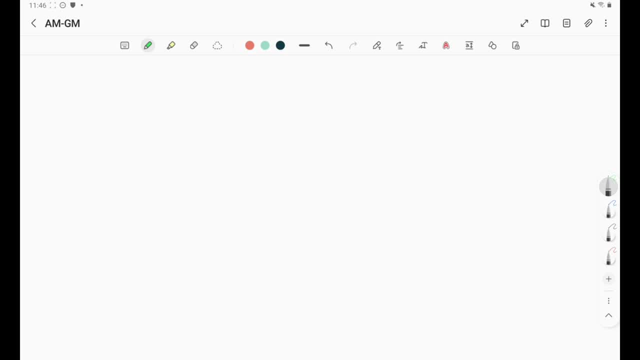 for example, the amgm, the couche-schwarz, the holder and all the famous inequalities, and of course, we the additional techniques and tricks that you need, and it will appear a lot in math olympiad contests. we will be dealing with all of that and the strategy for each lesson is simple. 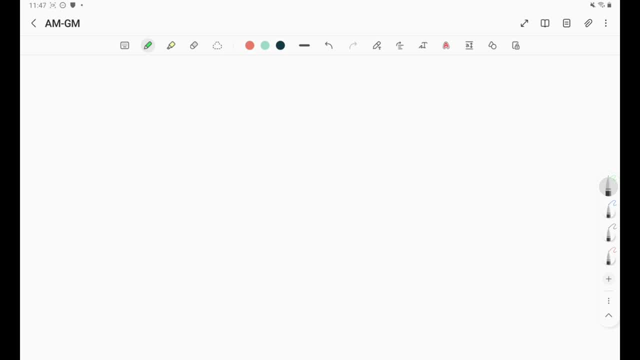 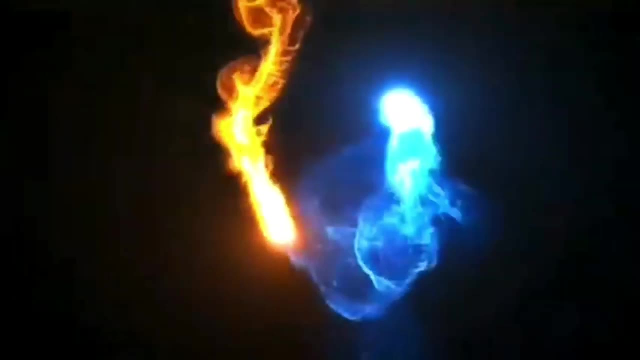 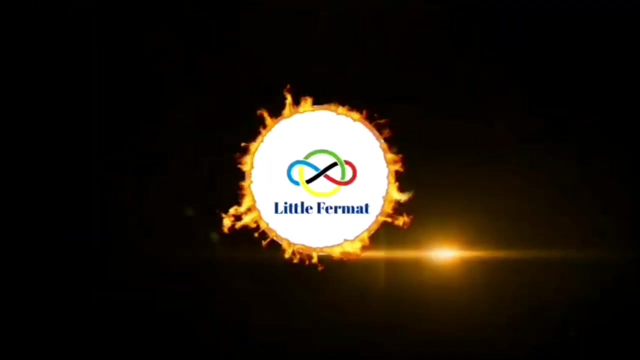 we'll just introduce the theorem, try to provide a proof, then go with easy examples first and level up until we solve IMO difficulty problems. so what are we waiting for? let's get started. before we start with our first lesson, I would like to talk a little about. 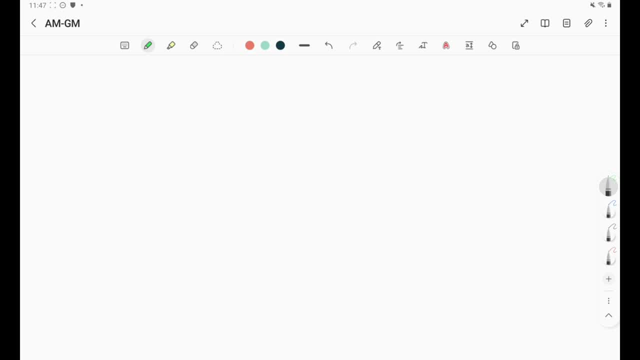 the history of inequalities in math, olympiad or the IMO specifically. so when the IMO started in 1959, inequalities were really important. so, like inequality history, special scores, benefits such as, went down every year. it questãoed other environmental factors, jupiter and psychology, when jupiter and chemistry were more importantoon. 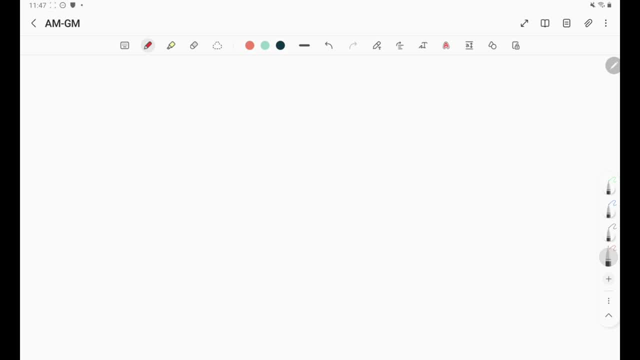 Like in each, like kind of in each year, we will expect one problem. Of course- like not necessarily each year, But, for example, if you just look at the first IMOs, you will see lots of inequalities appearing. So, basically, inequalities were really important. 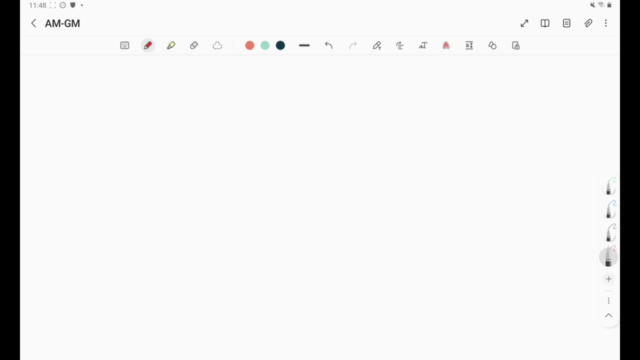 But later on actually suddenly inequalities disappeared from IMO. So if you just open recent years, like maybe 2010 till perhaps something like 2018, you will not see that much of mathematical inequalities there. Instead you will see just the algebra questions. 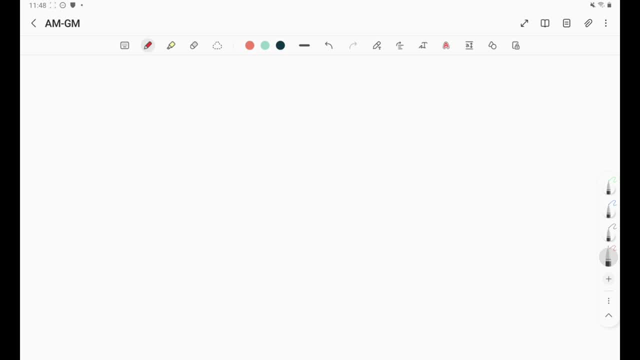 Most of them are either functional equations or like some other topic. So People really started ignoring training for mathematical inequalities And instead like we'll focus on functional equations or any other things like sequences or something else. But guess what? Just suddenly, in the recent years, inequalities appeared in the IMO. 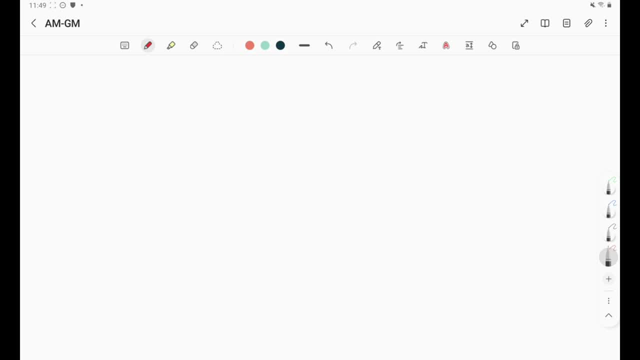 And like people or students were like caught by surprise as they weren't preparing that. So That's why I'm not going to talk too much for inequalities And hence, right now, if you are preparing for Math Olympiad, you really need to like develop your mathematical inequalities and just train on it, just like any other algebra topic. 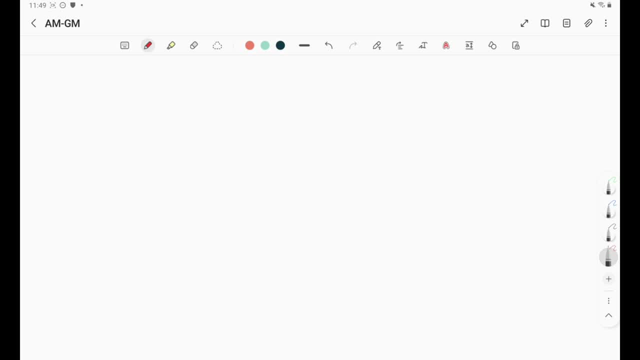 For example, functional equations or polynomials or anything like that, And that's why we'll simply begin by uploading this high quality Math Olympiad tutorial. So So, basically, our first lesson will focus on the AMGM, which is the arithmetic mean, geometric mean, inequality. 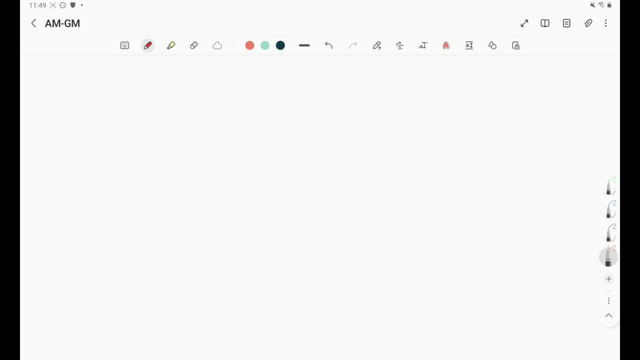 This inequality is really, really important And you usually will see all Math Olympiad books will start with this inequality. It's basically the core of the inequalities that you will see in Math Olympiad, So let's start by introducing that Before introducing the main theorem. I always like starting with a student. As I said, I always like starting with a student. I always like starting with a student at the start of the Math Olympiad And I like to talk about what I have done during my training And the number of questions you will ask about. 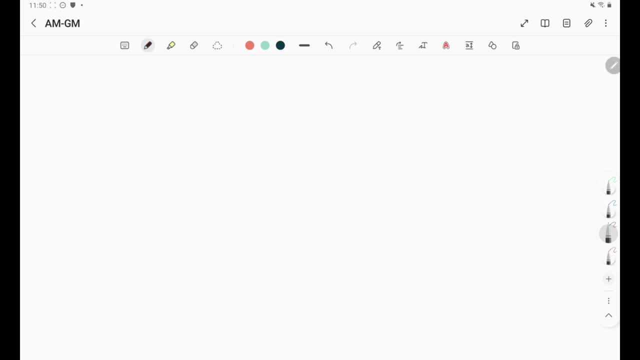 And because I'm a Data Science Professor, I have to do a lot of math on Math Olympiad. So this looks like a lot of questions related to my, my job, my knowledge that I do a simple example which is really simple: inequality, but it's like suitable as an. 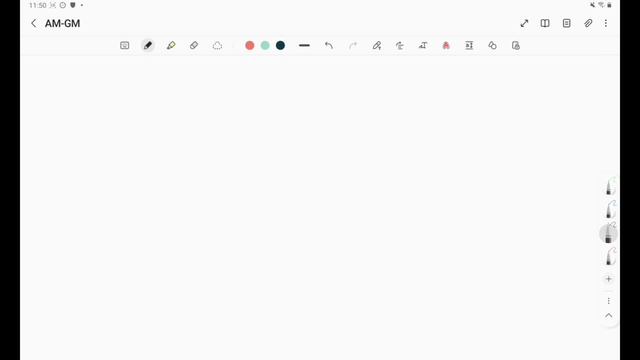 introduction. it's kind of a specific or a special case, a simple case for just two numbers of the AMGM. so let's say you want to prove for two non-negative numbers greater than or equal to zero, the following inequality: a plus b over two is greater than or equal to square root of AB. so give it a try and then. 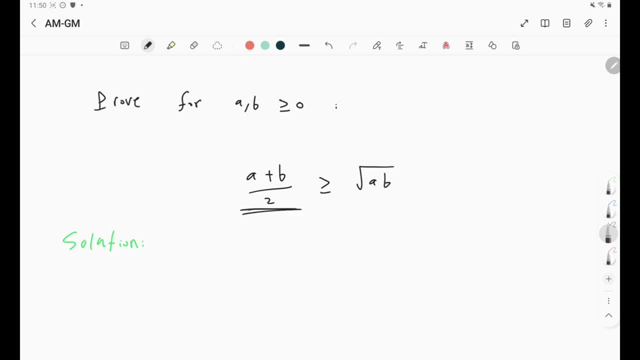 keep on watching. basically, this is on the left-hand side, is simply the arithmetic mean, as you can see: a plus b over two for the two numbers, and this is the б, the geometric mean, which is just the roots here. it's these like square root of the product, of the 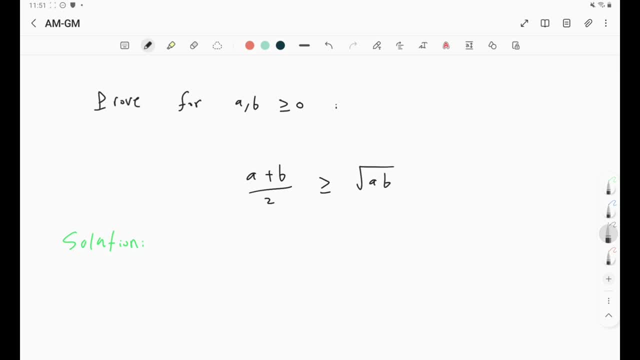 two numbers. so, as you can see, this is actually am- gm. the am is greater than or equal to the gm of the two numbers. but how can we prove this? well, first of all, let's simply multiply by two, both sides. so our inequality is just like this: a plus b is greater than or equal to. 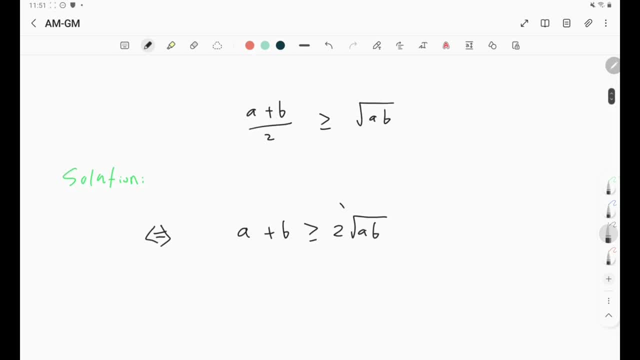 root a, b and of course, if we move stuff to the left hand side, this is the same as this. and if you just look at this, this should remind you of something nice. look at it. something minus two times: first number, second number, plus something like the second number, but of course here like we've got something squared, here's. 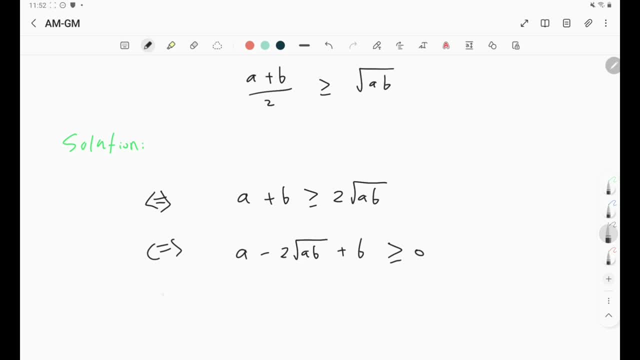 something squared. so this is simply the same as the formula root a minus root b squared. and guess what we're done? because, of course, any square number is non-negative, right? hence like the proof is done. of course, there is another way to prove this, which is simply like some people hate. 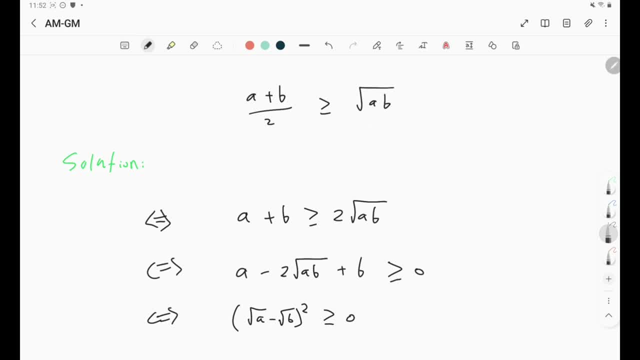 let's say roots. so they just end up squaring from the beginning, and this is not wrong. if you just square from the beginning, we'll also get the same thing, but of course we will get actually a minus b squared is greater than or equal to zero. so both both proofs work okay. so basically, as you can see, 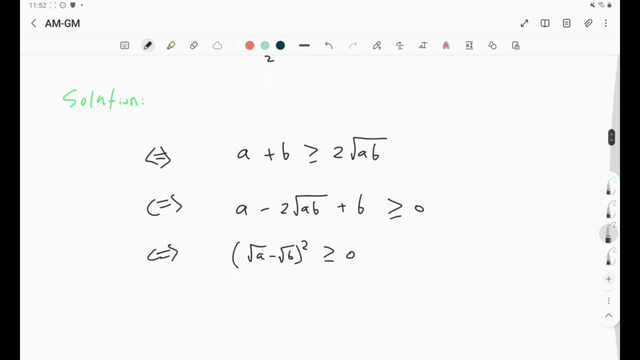 this is the amgm, just for two numbers. all right, let's actually solve one example, one problem on this before presenting the you main amgm. okay, so now we also want to prove, for three numbers that are non-negative, the following inequality: a squared plus b squared, c squared greater than: 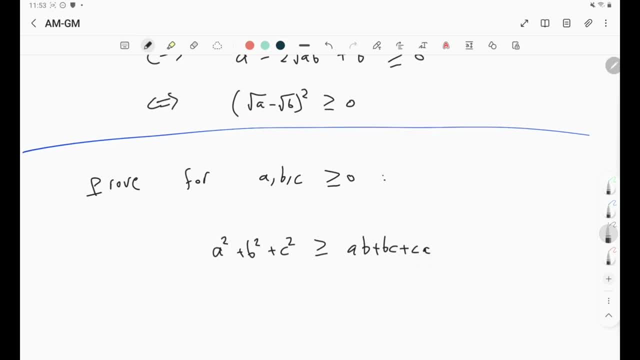 or equal to a, b plus b, c plus c. okay, before actually proving this, i want to really tell you some chords that for this amgm and joining the shower down over here we do only call one number. okay, three huge numbers and three said soon. sticker including six terms is equal. 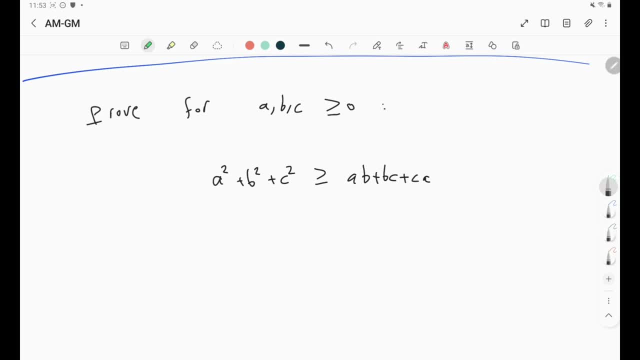 and so in that case you could put in in the opposite único of e, kosious as two, because there are no two standing. you need to rewrite every time that you putor in one word sigma or the sum notation. so, for example, let's say we have okay, here, three. 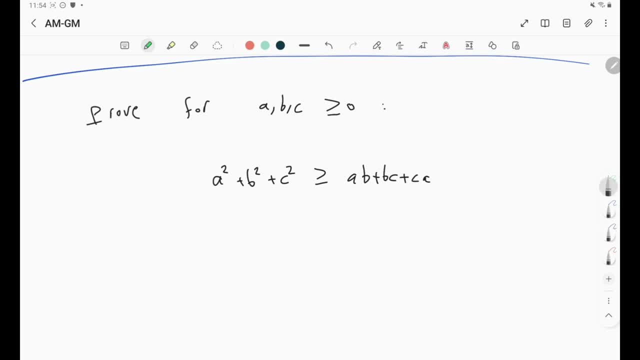 numbers a square plus b square plus c square, and on the right hand side we have a b plus b, c plus c a. do we each time have to write a square plus b square plus c square, and here a b plus b, c plus c a? actually no, you can use just. 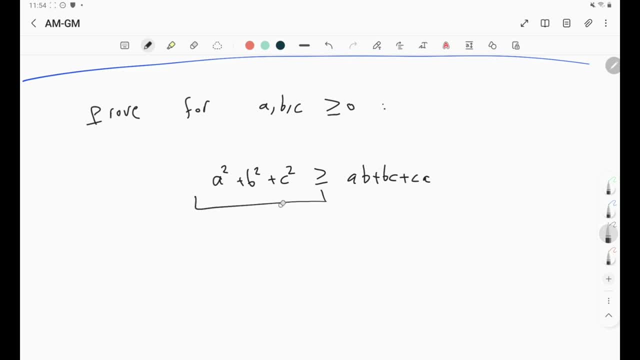 the sum notation, for example, we can represent the left hand side using sum a square, of course, like it should be clear that we just have three numbers, because maybe if we have just two numbers, it will be just a square plus b square, or if you have just four numbers, it will be a square plus b square plus c square. 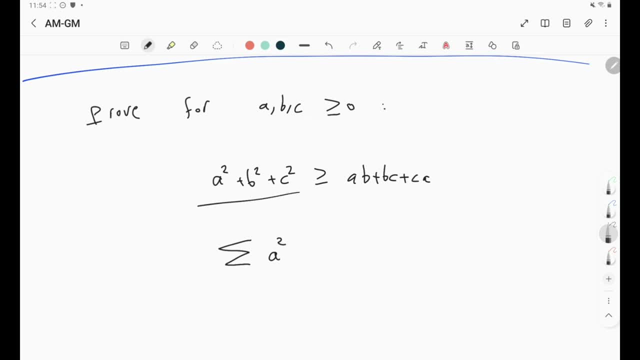 plus d square, so it should be really clear that we have three numbers here. then, of course, this sigma a square is just this left hand side. and what about the right hand side? you guessed it. it's just sum a ab. so you immediately go ab plus bc, plus ca. all right, so this is this will really be beneficial. 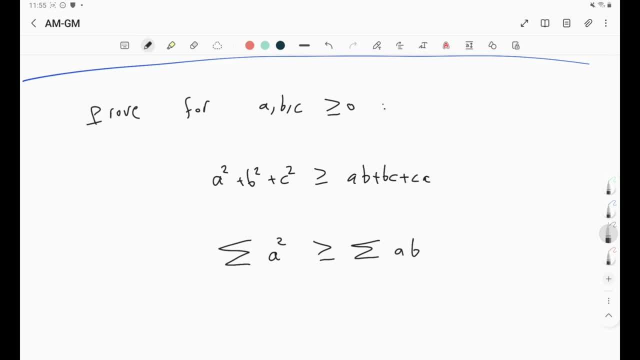 for us because it will save lots of, like, unnecessary writing and saves lots of time. so i like most of the times i'll be just writing sigma a square or sigma ab or something like that. of course, there is something that we'll also discuss which is like the symmetric sums and the 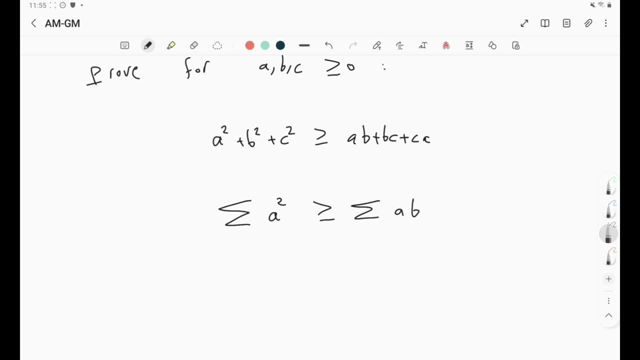 cyclic sums. okay, so if we want to explain it right now, shortly, basically, if we have something that is a cyclic sum, for example, let's say we have sum a square b and we say this is cyclic sum, what does that mean? of course, like we were working with three numbers, as we mentioned three numbers here. 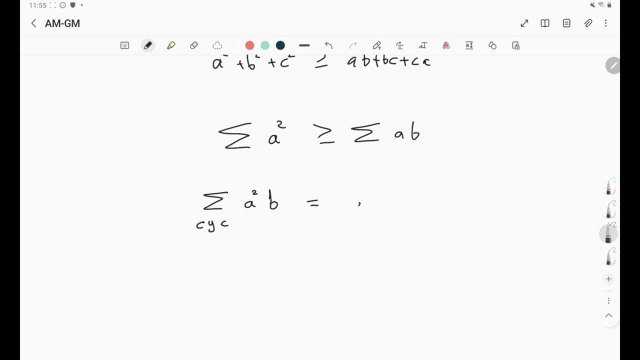 so we have a cyclic sum and we have a cyclic sum, and we have a cyclic sum and we have a cyclic sum that actually means this is a square b plus b square c plus c square a. what exactly are we doing? imagine that we have like a circle here and we have like kind of arrows going like this: 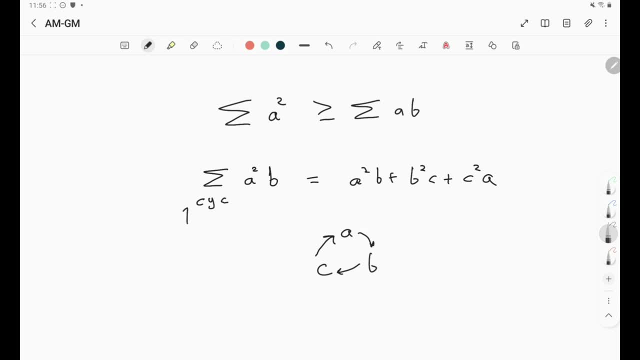 so okay, if we just look at this, what does it? what is it telling us? like, how can we construct that? this is this. why don't we have, for example, a square c? well, just look at this and you'll see that it's a cyclic sum and we have a cyclic sum and we have 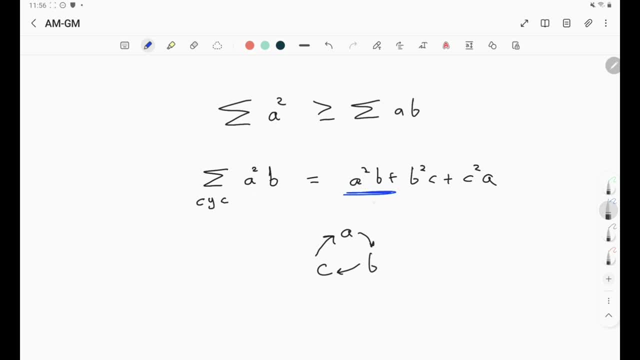 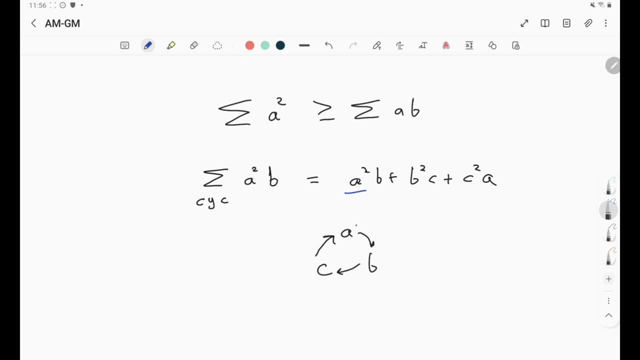 here we had a square b. next like a should be replaced with b, so we replace it with b. next after, in the like third, third term, we replaced b with what with c, so we've got c squared. so a square b, square c squared. same thing for 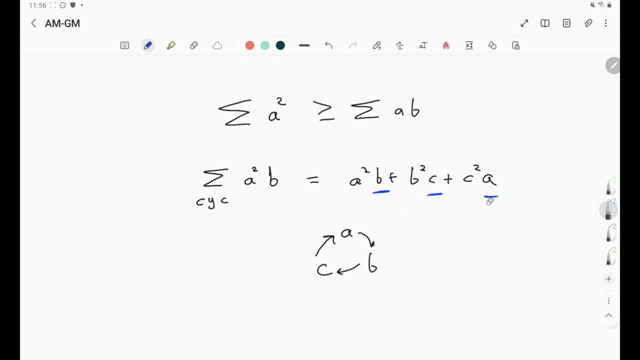 b. b is replaced then with c and then with a, so this is basically a cyclic sum by by the way, like if you, if you're using cyclic sum, you don't have to write cyclic sum. so if you, if i don't write anything, then you should automatically assume i'm working with cyclic. okay, then what? 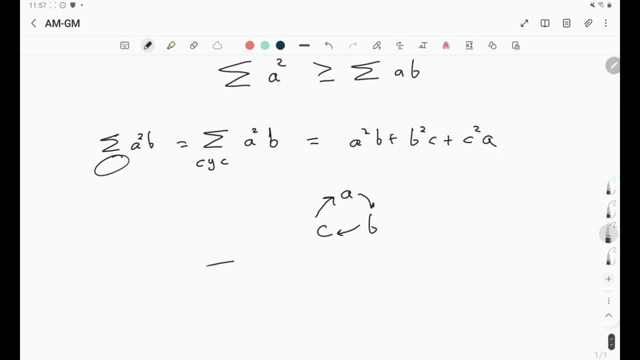 is actually symmetric sum. what symmetric sum is something different. if i write something like this, then it's not cyclic anymore. now i'll be using all different combinations. so now a square b plus a square c, like i'll be using everything. i'm not just going like in this circle, so i'll be using everything. a square. 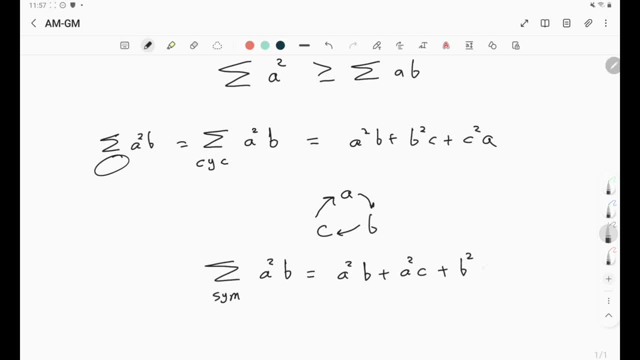 b a square c b square a b, square c c. square a c- square b. so it's really like obvious the difference between the like both of these. clearly, here the sigma symmetric has six terms, while the cyclic has only three terms. that actually makes sense here, because three factorial is just six and we're using all 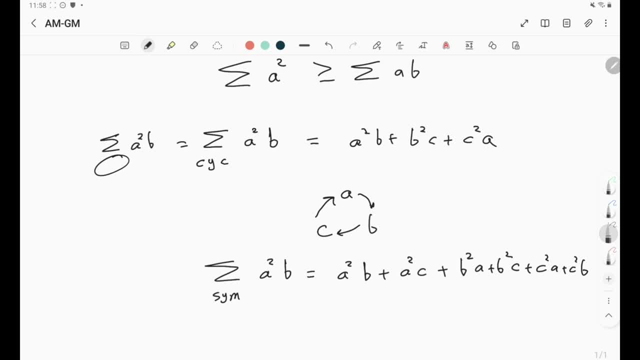 different combinations. so that's actually the difference between symmetric sums and cyclic and cyclic sums. so if if i don't write anything, then you should assume it's cyclic, but if i write symmetric, then like, of course i can't, like i need to specify it's symmetric. 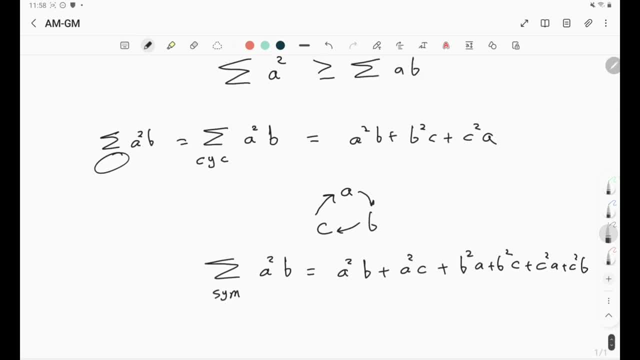 so that you understand what's happening. and also another thing: if i wrote sigma symmetric a square, then you should be careful, because this is not just a square plus b square plus c square. actually it is a square plus a square. so i actually like always, when, whenever you 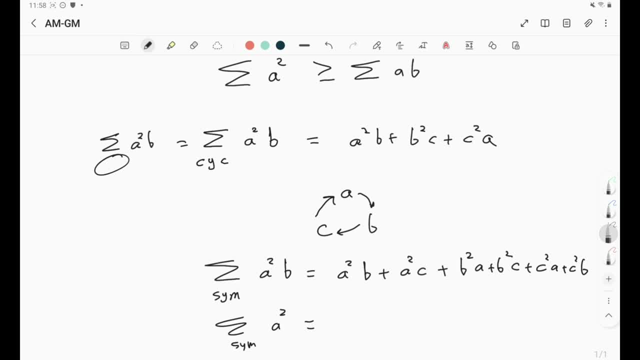 have a symmetric sum, then it must consist of six numbers, actually like six terms. so in fact, sigma's symmetric a square is a square plus a square plus b square plus b square plus c square plus c square, which is simply actually two sigma, a square, right. so as you can see here the, the sigma, 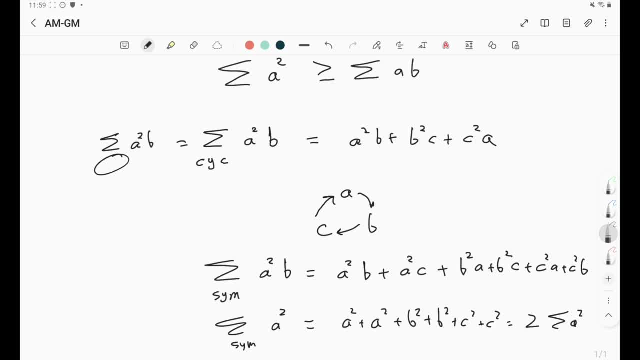 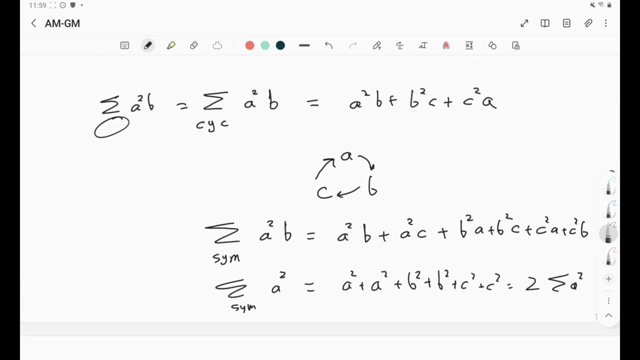 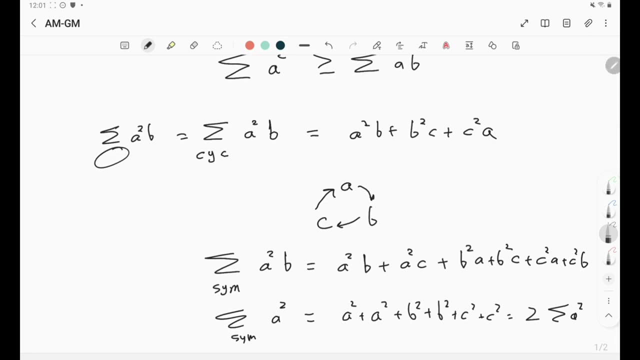 symmetric. a square is two times sigma, a square, which is cyclic. okay, so keep that in mind. okay, but that might be confusing when you start with it, but you should accumulate with it because you will face this a lot, so always keep that in mind. when you have a sigma symmetric, then you need to to cover all. 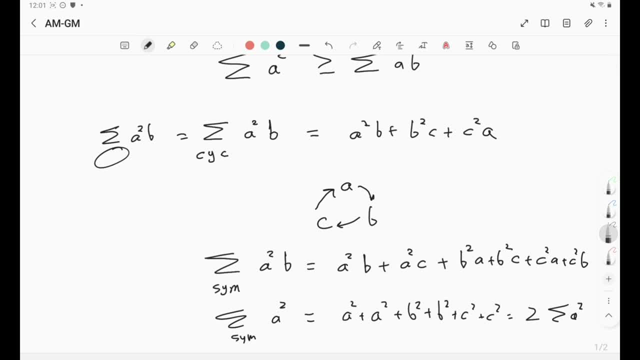 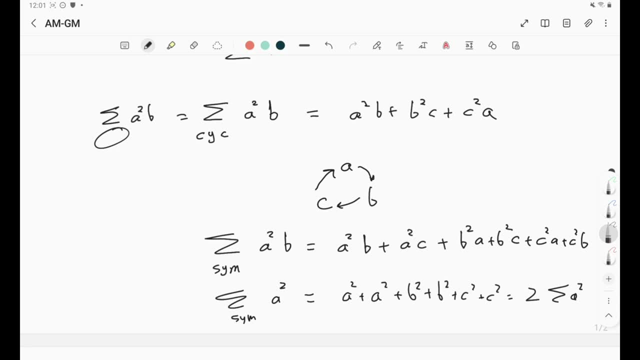 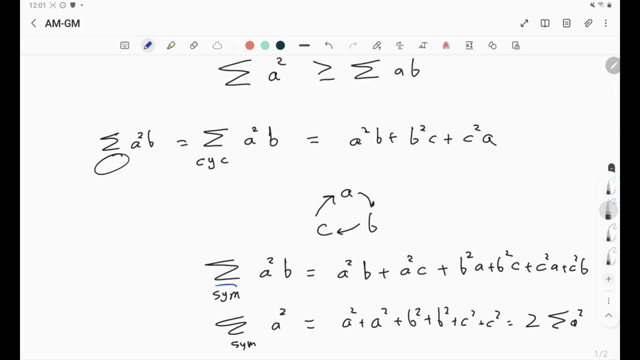 n factorial combinations, like you always have to have n factorial numbers or terms, of course. on the other hand, when you have cyclic, then you're just going in once, like a circle, so it's just in numbers instead, that in mind. another thing is that, of course, when i say sigma symmetric, it's different from: 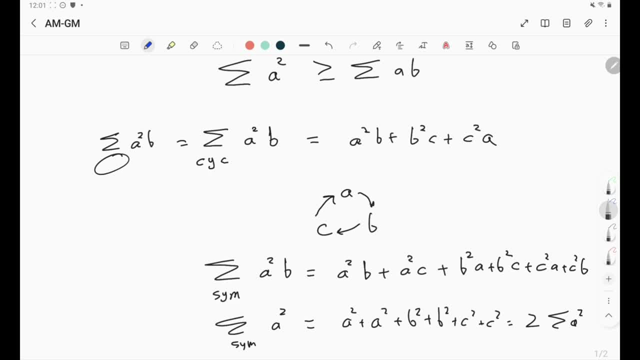 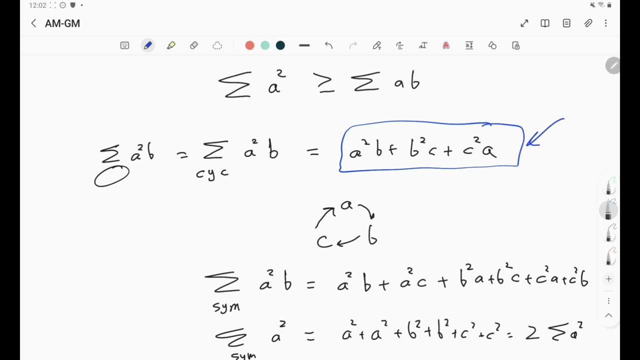 describing this, for example, like if you're working here, if someone asks you: is this asymmetric, is this, is this expression a symmetric thing? the answer is no, it's not symmetric because, as we said, like, we have a square b but we don't have a square c. so, if you like, write something like f. 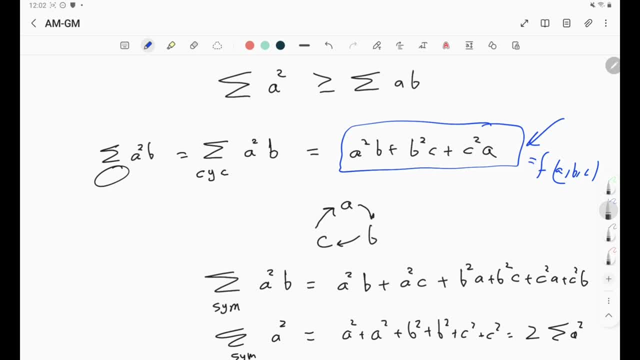 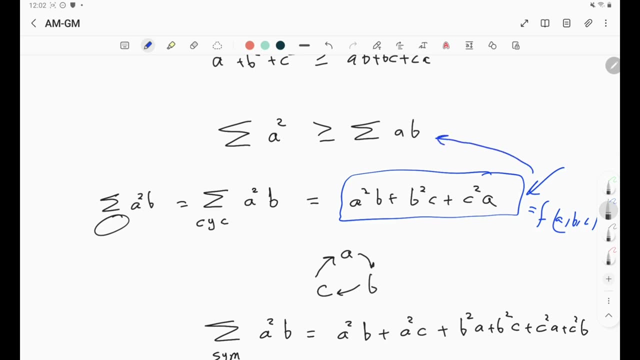 like as function f a, b, c, then the function f is not symmetric, it's cyclic. however, this one here: if you said f a, b, c is this, then it's symmetric. but what if i asked you this here: if we said f a, b, c is sigma a, b is it, is this one symmetric? well, you might say that no, this is a cyclic sum. 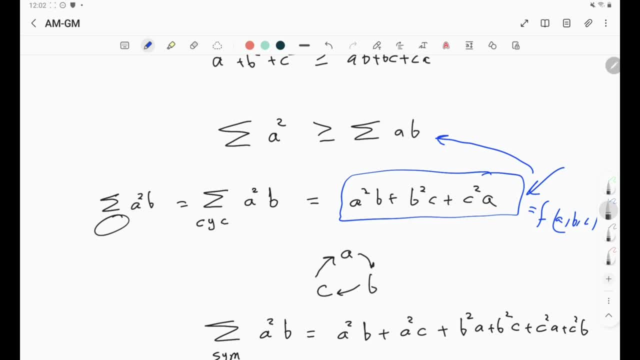 so it's not symmetric? but the answer is actually it is symmetric because if we're talking about the function, not the sigma, like here, we have everything we need. we have a b, we have b c, we have c a- all of them are covered. so the function f is. 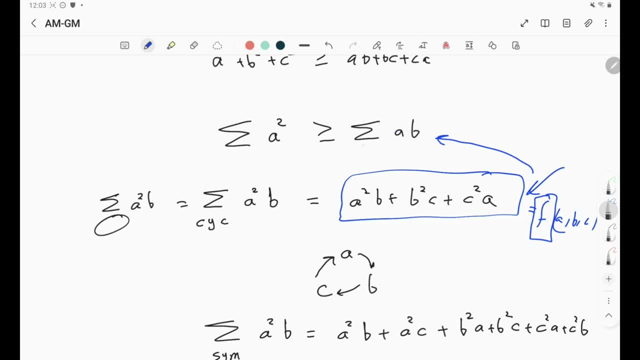 symmetric, but the sigma is not symmetric. like the sigma, if we wrote symmetric, it will be double, like two times sigma a, b. so it's a bit confusing, as i told you, but you really need to keep that in mind because it will be very important for us to to deal with like inequalities in general. 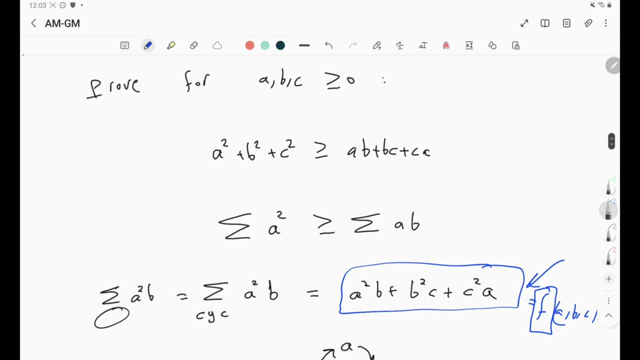 okay, so keep that in mind. so now let's actually just prove our inequality. let's write it again. now we just need to prove that. uh, okay, i'm not going to write sigma a square right now for like a certain purpose, as this is our like first lesson. 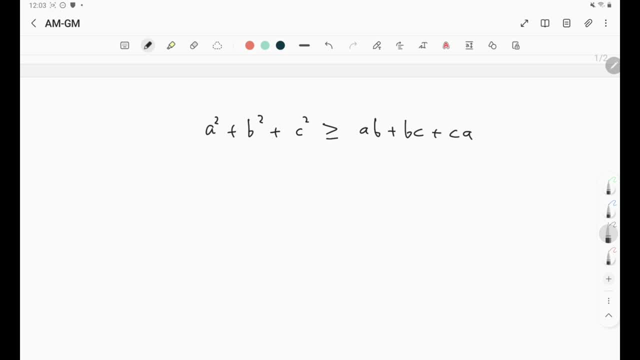 so i'll be writing, writing at all. so how can we prove this? as you know, we like the only tool that we explained. so we're going to do is: we're going to do a little bit of a test and we're going to do a little bit of a question requirement. we don't want to do it ourselves. make a test. 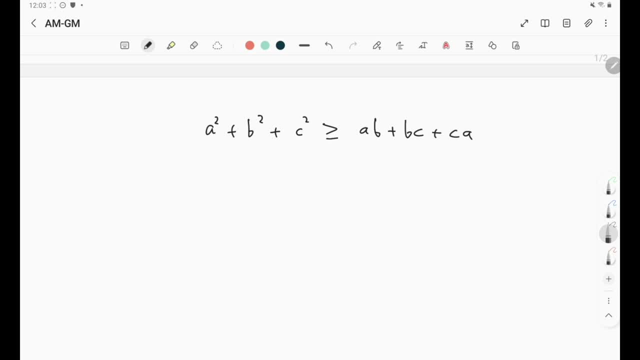 and on average it's promise. the most meaningful and the most прош sustained contribution so far is the amt m for two numbers, but here we have three numbers. how can we deal with that? well, we have actually a very, very powerful idea here. okay, you know what? let's just pick two numbers and try to apply the amgm on them. 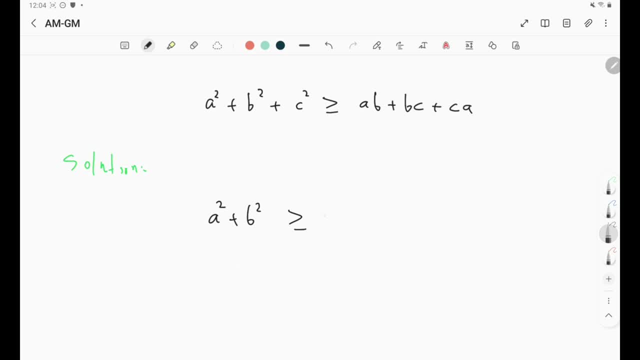 a b. in fact, like if you just multiply both sides by two, it'll be like this: now that's interesting: we have this one and this one, right, but we have a square plus b square and we have two a b. well, what happens if we do the same for the others, b square plus c square. so it's then. 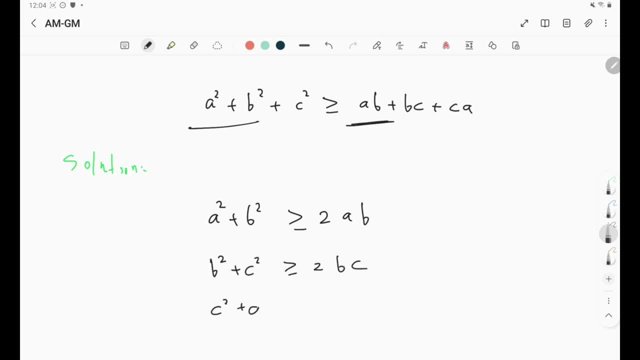 equal to two b, c and c square plus a square is greater than or equal to two c- a. guess what? now, if you just add these three inequalities, we're done, because now we'll get two. and now actually we'll get two sigma a square and here two sigma a- b, so basically we can cancel the two and get our. 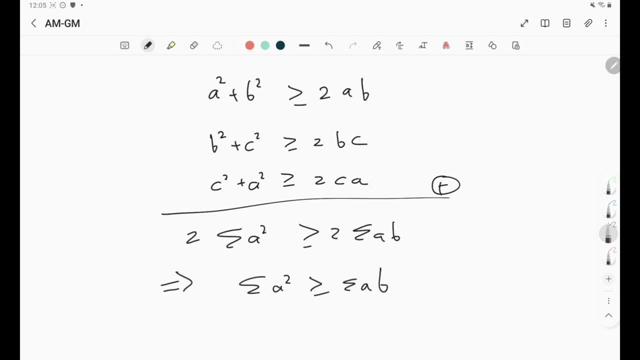 inequality. okay, so this technique is really powerful, like it's kind of uh called the pairing technique, because we're pairing, like, okay, we need to get a b, how can we get a b? you need to get pair a and b. so if we pair these, we got a- b. same thing for each. like b, c. 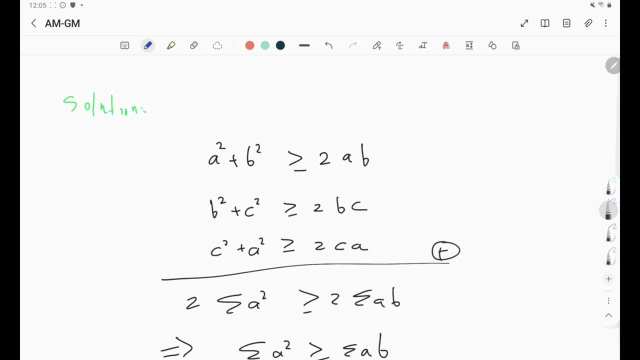 we are these, we got it like. you should always believe that once you get one of them, then like, of course the others are, are the same, and then if you just take the like, the sum of them, you're done. like you, you must be done, don't worry about it, just worry about, uh, like getting, let's say like, 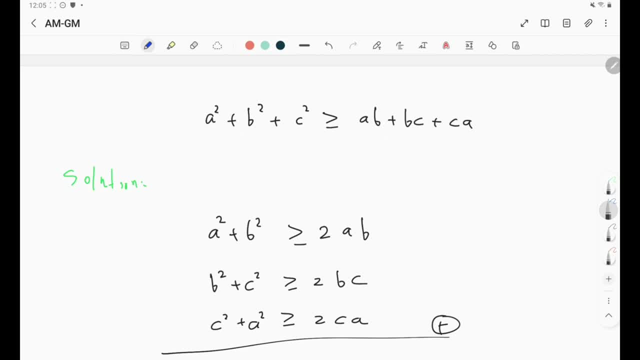 pairing them up and and getting rid of of at least one. okay, so this strategy is really powerful. by the way, like here, we applied the amgm for two numbers, but it's not on the roots because we have them squared. so i really like, want to write here these two versions of the amgm. so version one: 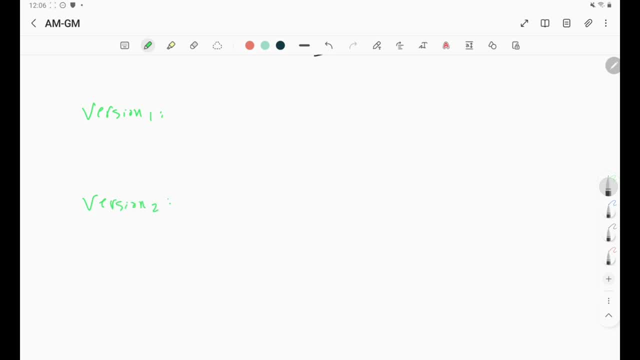 and version two, just for two numbers. we haven't, like, presented the amgm, the actual amg, so for two numbers we can write this: a square plus b square is greater than or equal to two a b. we already just do it like i did that, because of course a minus b squared is greater than equal to. 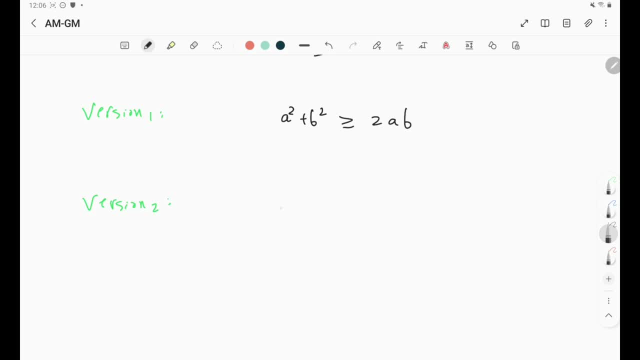 zero. yeah, the other version is actually the same as amgm, remember like we know this. so what happens if we square both sides? we'll have this right, okay, so these, like two, seem like the same. however, they're a bit different and each one has its own. 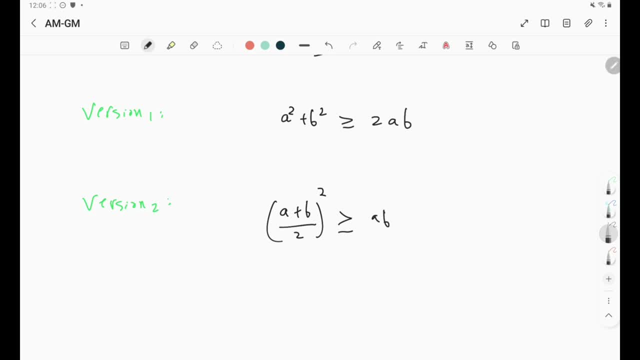 usage. it depends on the problem because, for example, let's say, in a question, they told you that a plus b is equal to 2.. then, uh, here you know that a, b is less than 1. you will not apply this. you apply this. but what if they told you that a squared plus b squared is equal? let's say to: 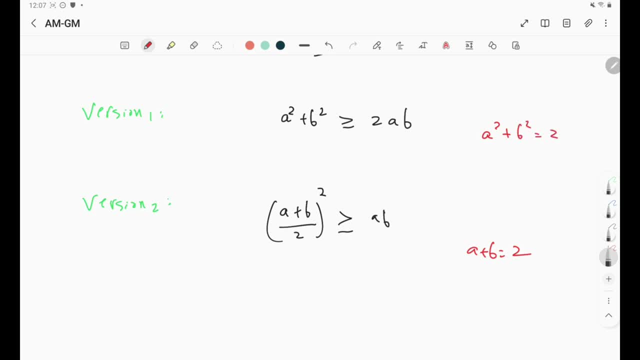 four like equal to two, then of course you'll apply the first one, okay, so then keep that in mind. we have two versions: one links a b to the sum and one links it to the sum of squares. okay, so now let's move on and present the real amgm, the generalized version. so 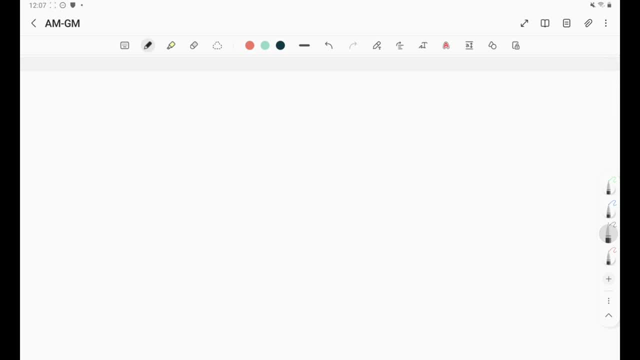 the generalized version is the following: let's say we have n numbers, a1, a2 up to an, and they are non-negative numbers. then we have the following inequality: a1 plus a2 till an. we said it's the am right, the arithmetic mean or the average. that's it. what is the geometric mean? 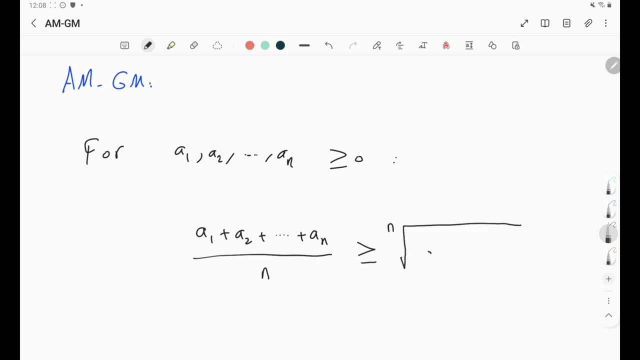 a1 plus a2 till an. we said it's the am, right, the arithmetic mean or the average, that's it simple. the nth root: the product. okay, so the am is greater than or equal to the gm, that's it okay. so actually, as as we mentioned, we'll be dealing with sigma. 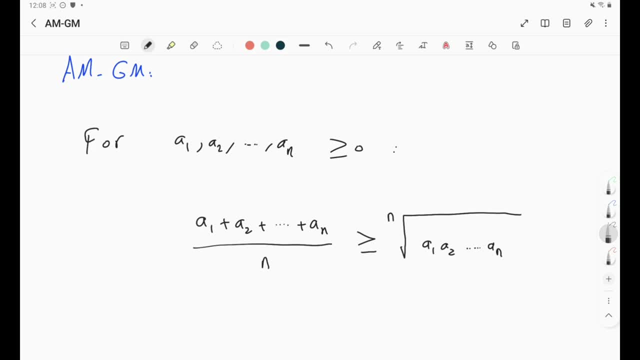 like, in order to cancel time, we don't really want to, uh, spend lots of time each like writing all of them, and you're also writing all of them, so let's write it in a simpler way, using the sum notation. so, for example, the, the lhs is actually sum a, i going from one till n. 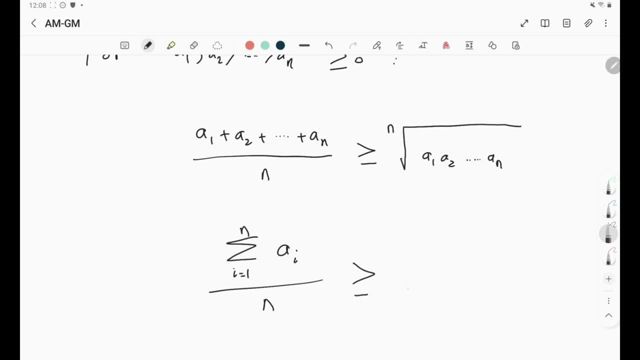 over n, of course, and the right hand side, actually the nth root. okay, we don't want to use, like the product, a1, a2 up to a n, so we'll just use the pi symbol. so the pi is the same as product, of course, going from one till n, okay, perfect. so this is also the amgm, i think, with just the. 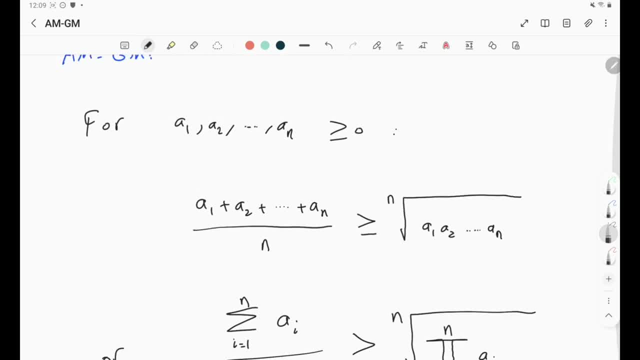 symbols. okay, so of course, some some notes here. the numbers must be non-negative because of the roots pink. you need to keep that in mind and, like in general, you need to apply amgm, the. the numbers must be non-negative because of the roots pink. you need to keep that in mind. 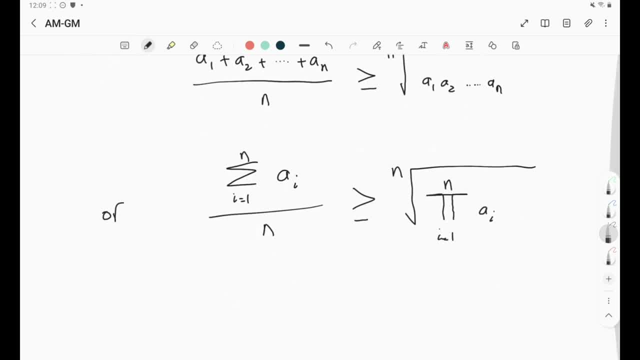 numbers should be non-negative because in some situations- let's say you, you, you're applying it for three numbers. you're saying this: if the numbers actually are all negative, it will be reversed the the reason is simple, like i'm not sure if you know this, but keep this in mind. this: 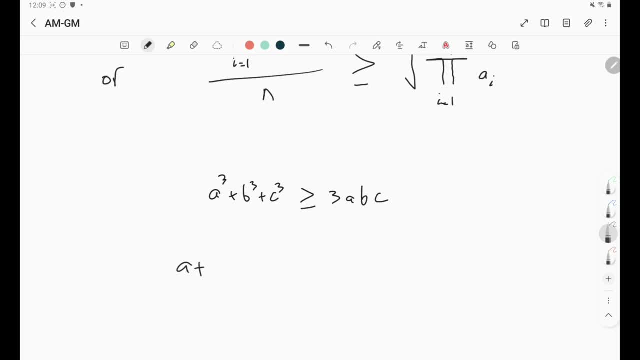 is really a powerful algebra, like a trick that is very powerful. the this: this can be factorized. if you move this to the left hand side, you can factorize it. so: a cube plus b, cube plus c, cube minus three, abc, this is just the sum of the numbers times. 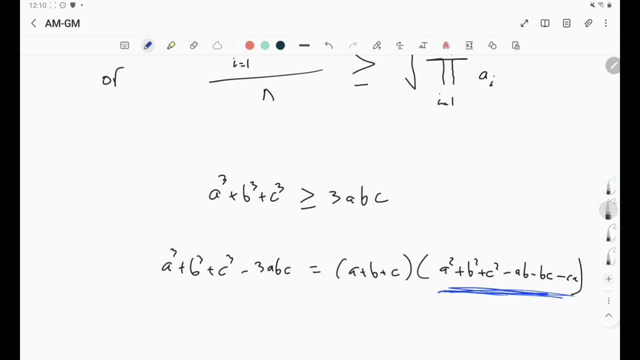 so what does that mean? remember, we already worked with this. we said it's always positive. this is all always positive. actually, even if it was like the numbers are negative, all of them are negative- this is still positive and i will leave it to you to check why. like, try to work with this and see why it's always 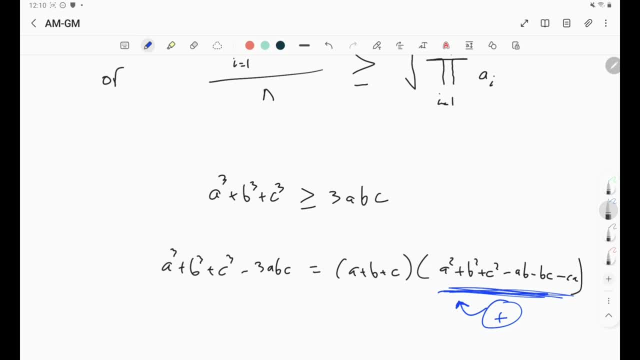 positive. even if the numbers are negative, try using the same as our proof. but if this is positive, then that means this: the sign of this is the same as the sign of this. so if all of the numbers are positive, then okay, the amgm works for three numbers. this is positive. this is positive. so, as 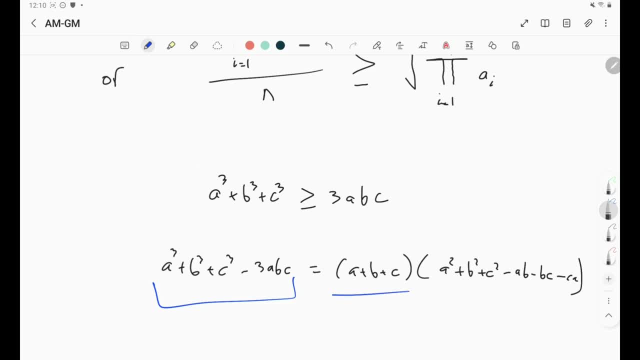 indeed this is correct, but if the all of the numbers are negative, this is negative. of course, if you add three negative numbers, you'll get a negative number right, so this will be reversed, and hence you need to to always remember you cannot apply amgm if the numbers are negative. 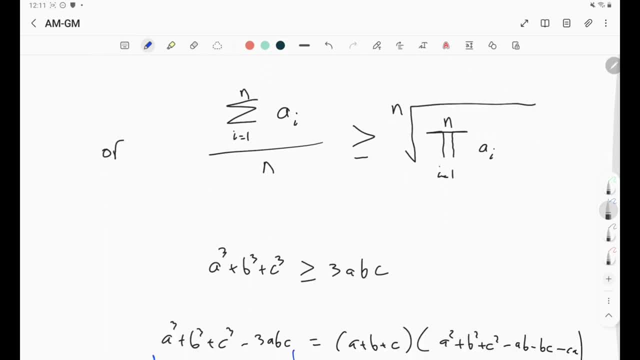 keep that in mind, generally speaking, of course. okay, so this is the amgm. how about we give it a proof? of course, there are lots of proofs for the amgm, as it's really famous, but we will just pick one that's really nice. we'll basically pick an idea using induction. 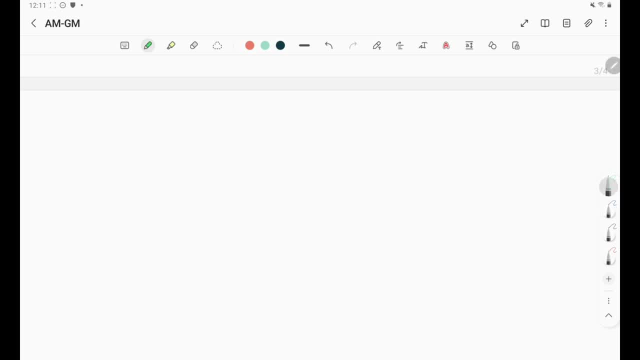 however, the proof that we'll be discussing is not an ordinary induction. for example, you might be familiar with the induction going from n minus one to n. the induction that we'll be working with is not that this unfortunately doesn't work. you can try with it. we'll be using. 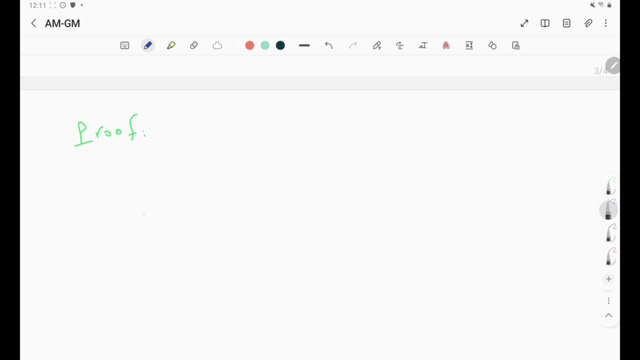 another type of induction which is really kind of weird, but it's really nice. we'll be moving from n to 2n. wait a minute, how are we going from n to 2n, like even if we can do that? so one will lead to two, this will lead to four, this will lead to eight, sixteen and so on. any power of two right. 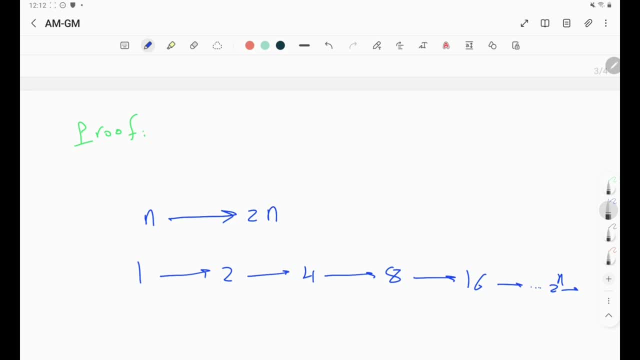 okay, that that doesn't. that doesn't solve the problem, right? we've only proved it for powers of two. well, of course this is not the whole proof. this is only the process one. let's say we have another process which is going down from n to n minus one. so, for example, now how can we cover three easy? 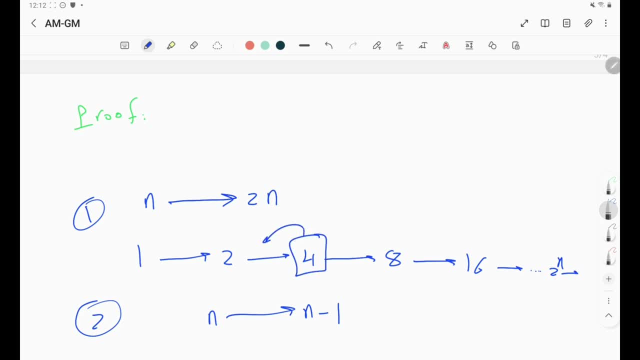 because four is correct. you can use process two to cover three. how can we cover five? well, easy, from eight we can cover seven, and seven covers three. so we have another process which is going down from n to n minus one. six and six covers five, and so on. in fact, likely that means process one, the only uh like usage for. 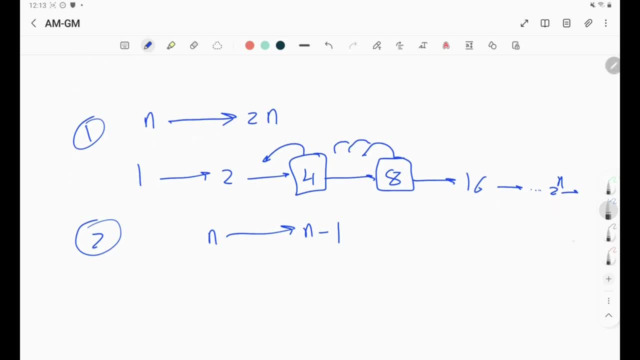 process one is just to give us, like the big values, right, like if we go to infinity, then we use process two to go down to one. so this idea is really cool and, uh, let's see how we can prove the mgm using this idea. so first of all we'll begin with the first, let's say first idea first. 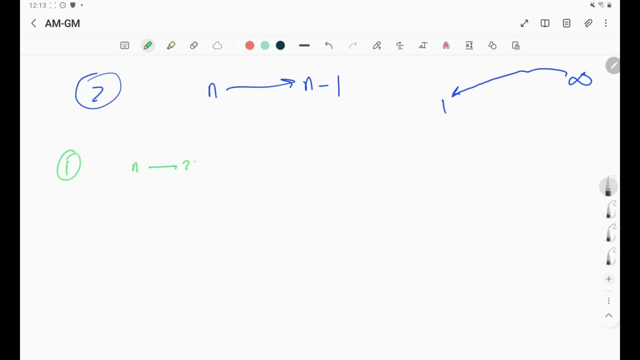 process move like proving n to 2n. so we'll assume that the mgm is correct for n numbers and we'll be working with 2n numbers, of course, like working with n equals one. uh, it's really like simple n equals one and two. so we'll just be working with n and proving it for 2n. so let's do that. 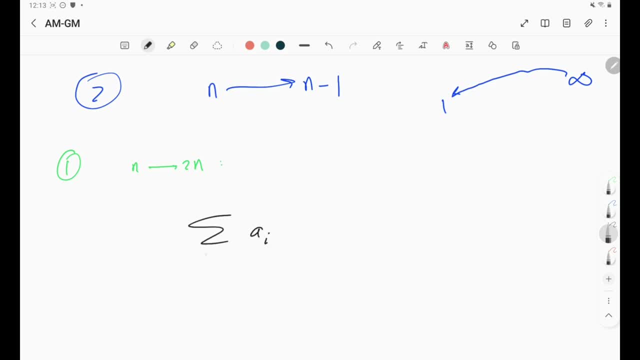 we want to prove the sum of ai's going from 1 till 2n. over 2n is greater, uh, greater than or equal to 2n. root pi ai from 1 till 2n. okay, i don't need like each time to write like i, because it's really clear. 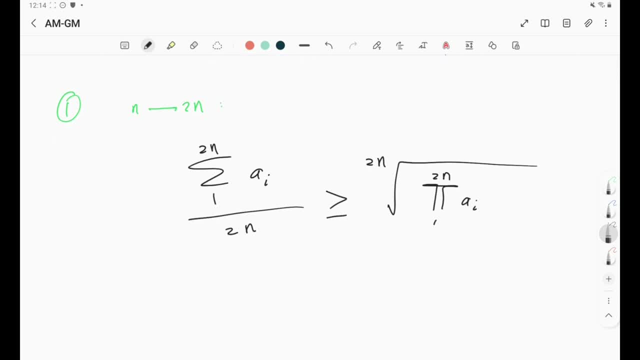 so how can we prove that? of course we need to use uh, like the, the n, the n case. so we'll be working with n numbers and another n numbers. we'll simply split it into two sums. uh, okay, this is easy. so this is equivalent to going from 1 to n and then from m plus 1 to 2n. 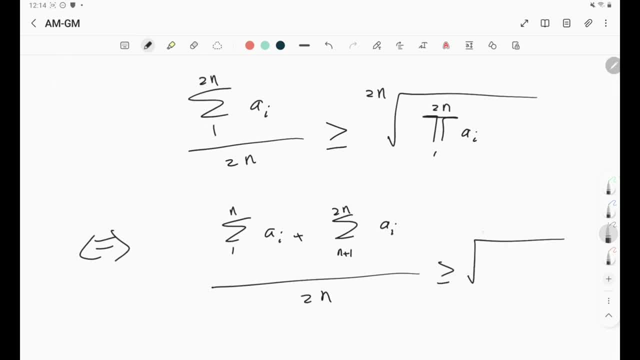 and all of that over 2n. and you know what? like, let's work from left hands, from left, like just this is the lhs and try to apply the amgm because, remember, we can apply it on any n numbers, so we can apply to here and here. okay, 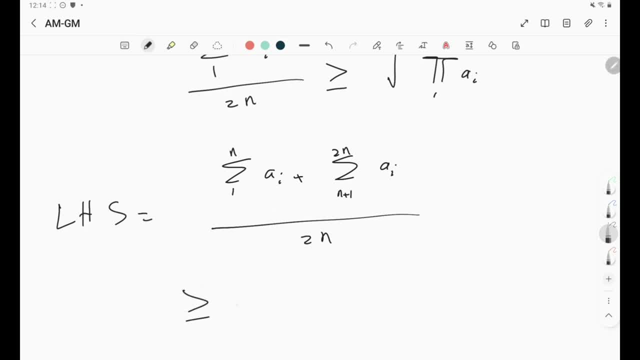 simply, we'll be applying it. so if we apply the amgm, then here we have uh n times nth root product ai from 1 to n, and here another n times nth root pi ai going from m plus 1 till 2n. all of that is divided by 2n and now, of course, the end. like the end cancels the end. 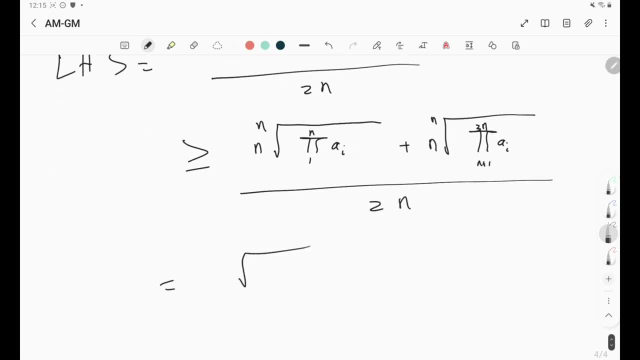 so now, actually, this is just equal to plus this over 2, of course, going from 1 to n and from n plus 1 to 2n. now, actually, if you think about it, how can we go from here, from here, to what we want here? the idea is really simple, remember. 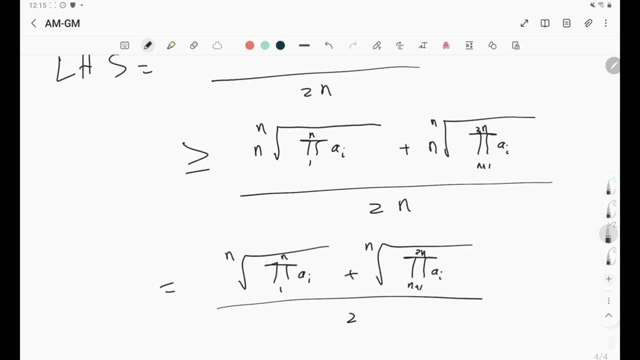 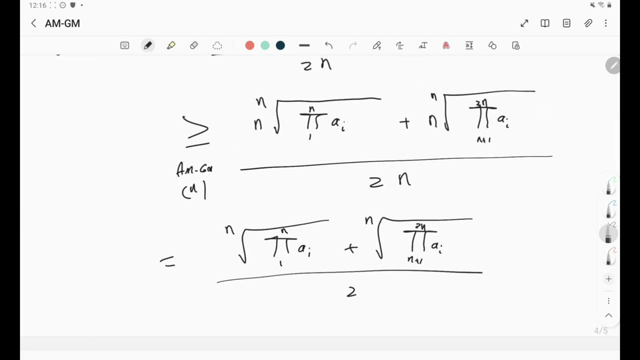 here we have a 2, so why don't we apply the amgm only for two numbers? right makes sense. so if we apply amgm here for two numbers, here we applied amgm for n numbers. but now, if you just apply that the two will cancel the two, because 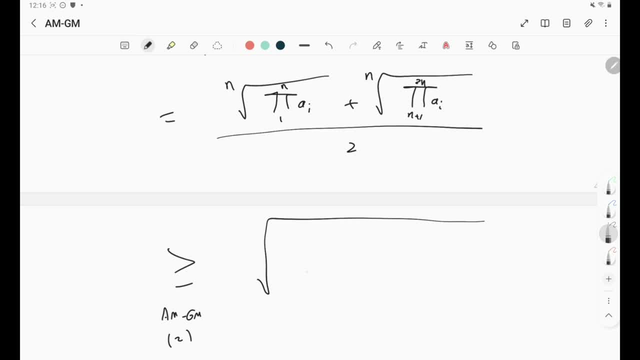 this is the arithmetic mean, so we just have a big square root of this. so from here we can see that this is going from 1 to n and we're going to apply n times this. okay, so now we're going to apply the arithmetic mean, so we're going to apply n times this. 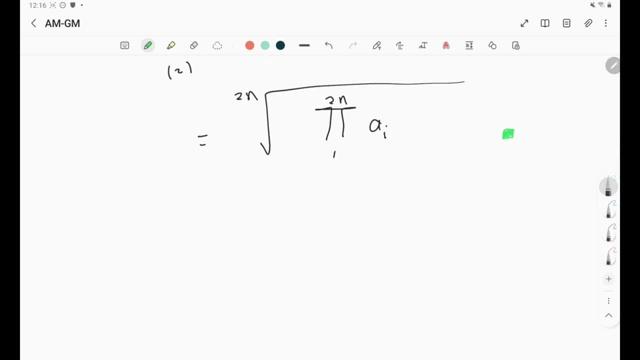 okay, this is what we want. Let's go for process 2.. So now we want to go from n to n minus 1.. Alright, now, if you think about it, we need to prove it for n minus 1 numbers, But we know it's true for n numbers. 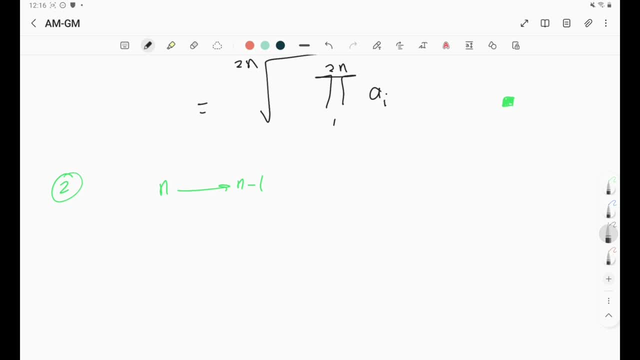 So we want to start with n numbers, But one number should be kind of fake. It's not a new number, It's kind of a function of the n minus 1 numbers. So, if you think about it, what should we use? 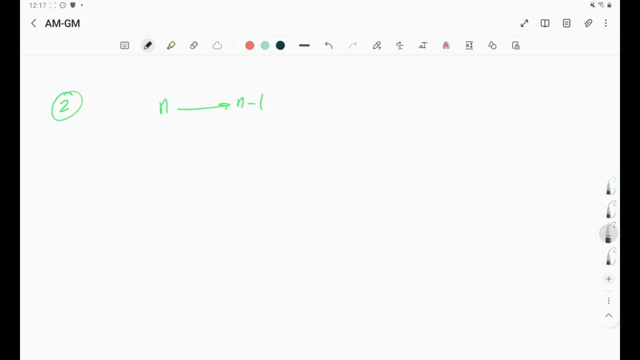 Generally speaking, in inequalities, what is the useless number Like? the number that doesn't affect the inequality that much If you think about it, it's usually the average. The average actually doesn't change the quantity that much. right, So this will be our strategy. 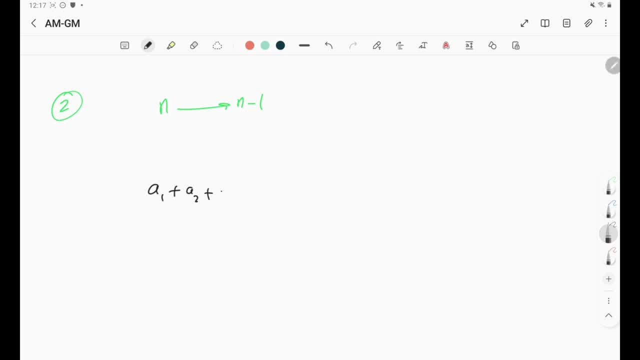 So we'll be putting the numbers. These are the n minus 1 numbers. But what is the nth number? It's actually the average. So here the nth number is just the average. So guess what? Let's just write it using the sum notation. 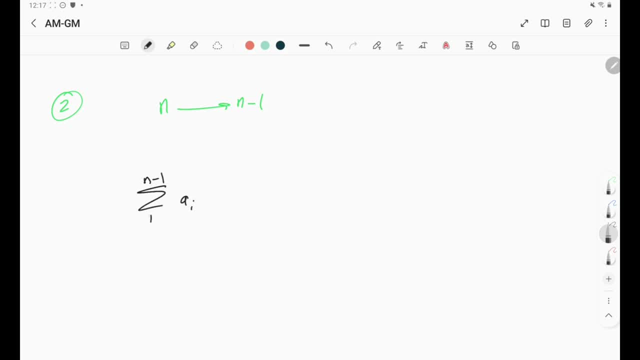 From 1 to n minus 1.. These are our first n minus 1 numbers And this will be our. This is our nth number. Okay, remember, it's correct for any n number, So we'll be applying that. So here over n is greater than or equal to the nth root. 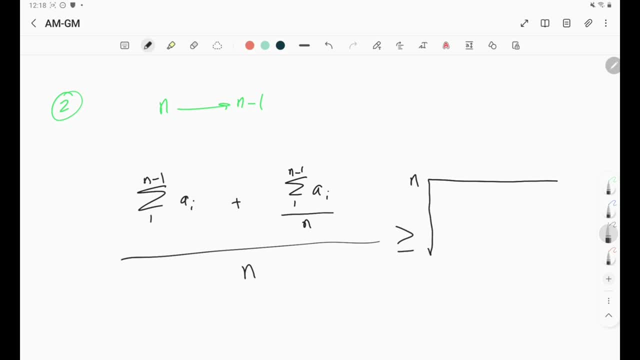 Here you need to be careful. Why? Because Remember what are our numbers: a1,, a2,, a3, up to an- Sorry, an minus 1.. So it's actually pi of ai's From 1 to n minus 1.. 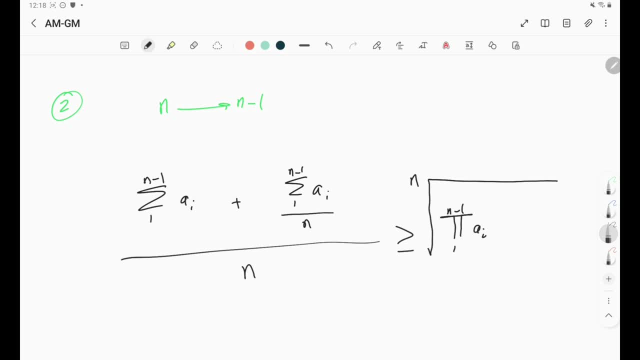 But now what is the missing thing? It's the nth number. And what is the nth number? It's all of that. This is one block. This is one number. Don't be fooled, It's not like a sum of numbers. 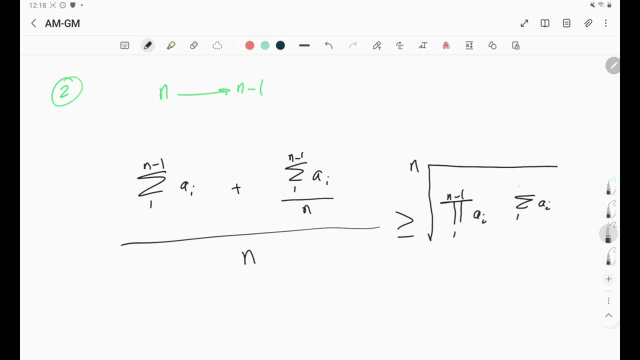 So I'll just be putting that, All right. So I know this is true And I hope to show it's true for n minus 1.. So, basically, let's simply do some algebra Because, as you can see, this is here, here and here. 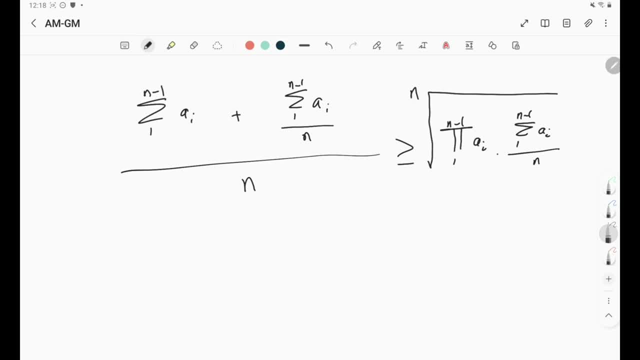 So probably we can use some algebra tricks to play with that. So the left-hand side, if you take this as a common factor, you can take this outside, And now we just have one. Oh, actually, sorry, I made a mistake here. 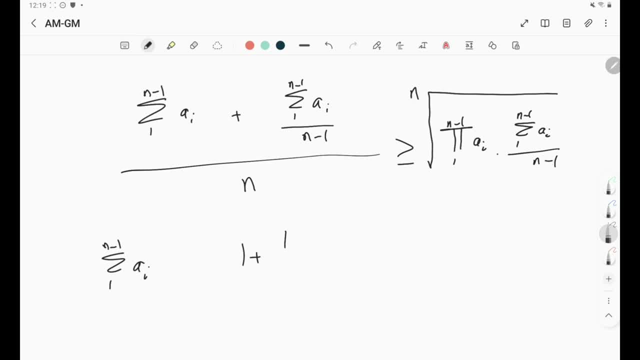 This should be n minus 1.. Here it's n minus 1.. Because we said that this is the average right. So okay, Keeping that in mind, what is this? This actually is just n over n minus 1.. 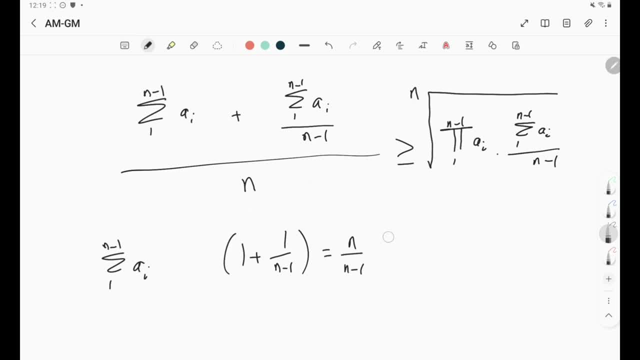 But okay, that's cool. n cancels the n, So we just have over n minus 1.. All right, perfect. So let's immediately write it Over n minus 1.. This is the left-hand side, The right-hand side, it's still. 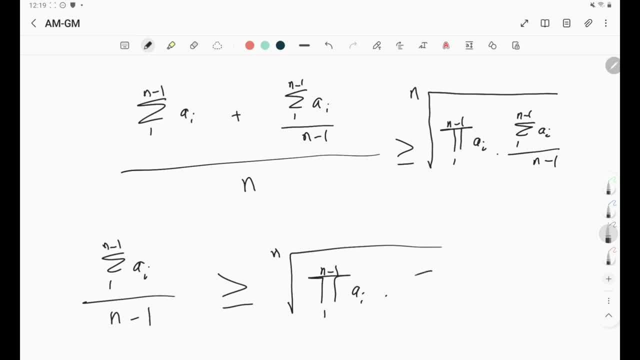 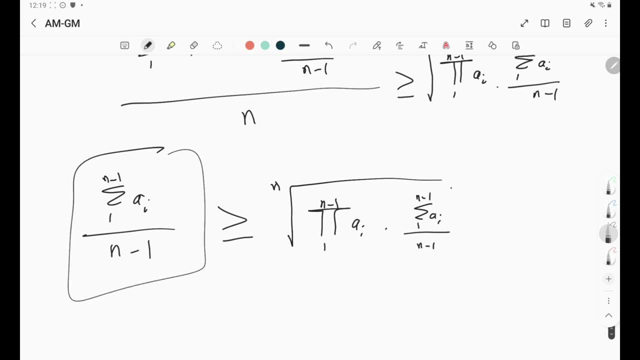 This times this. Okay, Now also we have something nice. This and this: they are the same, So let's cancel them, Okay. it's a bit confusing how we can cancel that, having the nth root here, So we'll just simply take both sides. 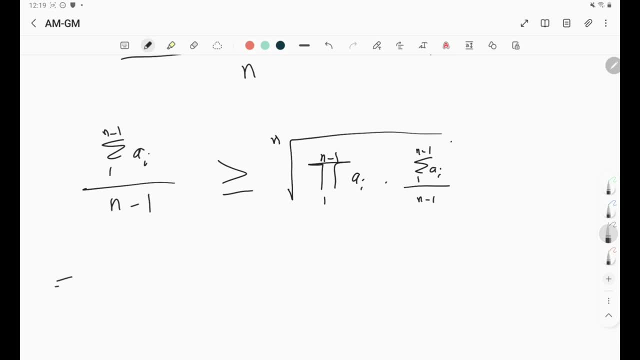 and raise them to the nth power. Okay, so now this is To the nth, And now we remove the root here. Okay, perfect, So now we can just cancel that. Okay, I'll be actually doing it from here, Just here. 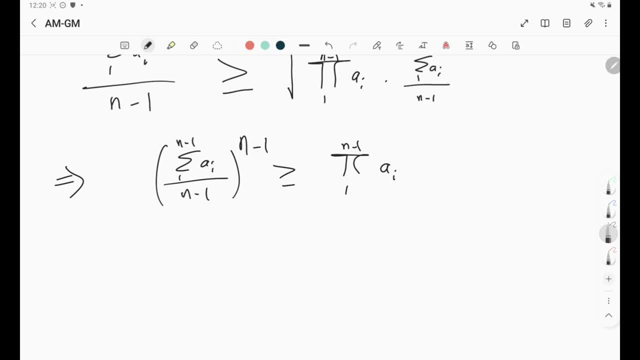 I will be erasing this. Okay, perfect. Now what's the only thing that we need to do? Notice that this is really the amgm that we are looking for, But we just need simply to take both sides to the n minus 1th root. 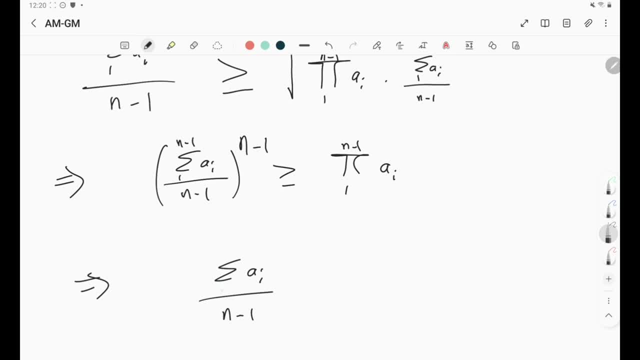 And we'll be done. Notice, this is the average, the arithmetic mean, And this is nothing more than Nothing but the geometric mean. And we're done, All right, perfect. So that means That means We have shown the process 1 and process 2. 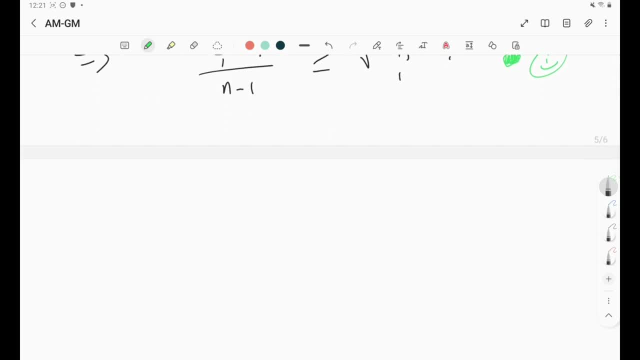 and hence, using induction, we're done. We can simply like go to a very like big, big number, And then we can, using process 2, we can go till 1.. Okay, perfect, So we've proved the amgm. 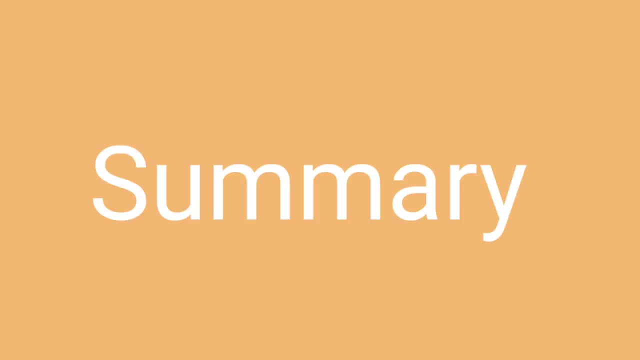 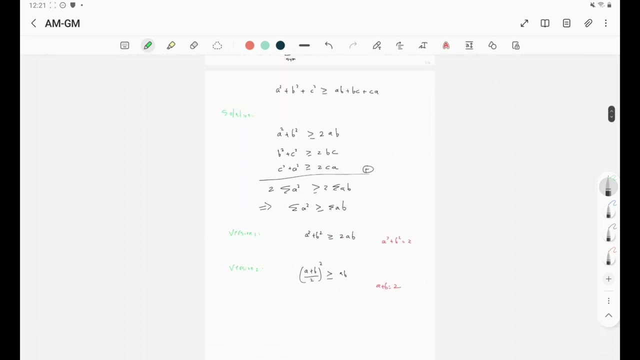 And that actually is enough for our first lesson. All right, so in this lesson we learned about the kind of. We took an intro to inequalities, We said that The amgm is really powerful in equality And we just provided the amgm, first of all for two numbers. 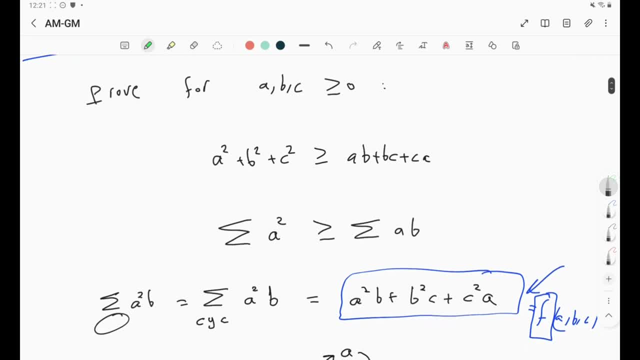 And then we took a special case- or sorry, like a special example- on just the two numbers. We learned this technique of multiplying both sides by 2 and pairing stuff up, pairing things up as we did, like a squared plus b squared with 2ab. 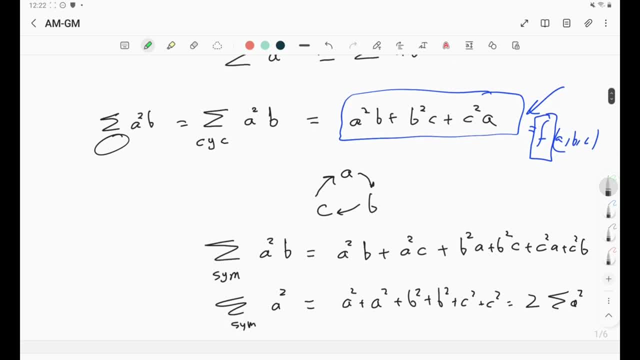 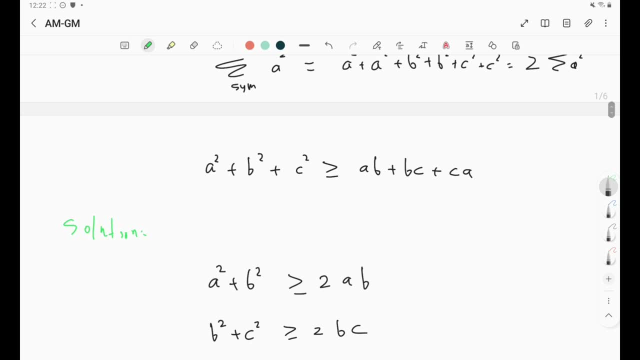 And we also learned about the cyclic sum, the symmetric sums and- like I really want you to understand that because it's very important in your mathematical inequalities journey- And we also discussed the amgm, basically the main theorem, the generalized theorem. 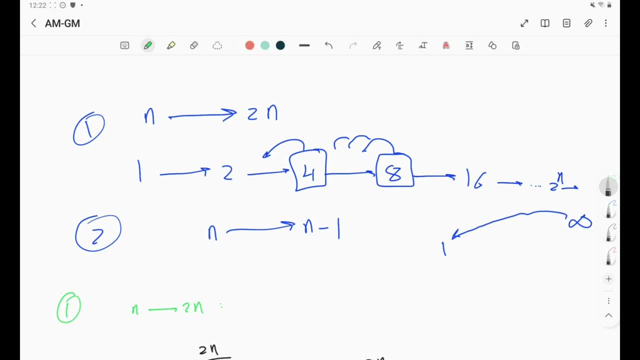 And of course, we proved it using this nice induction proof, like going from n to 2n and from n to n-1.. Just one thing I forgot to tell you. That is the equality, The equality case in the amgm, like in each inequality. 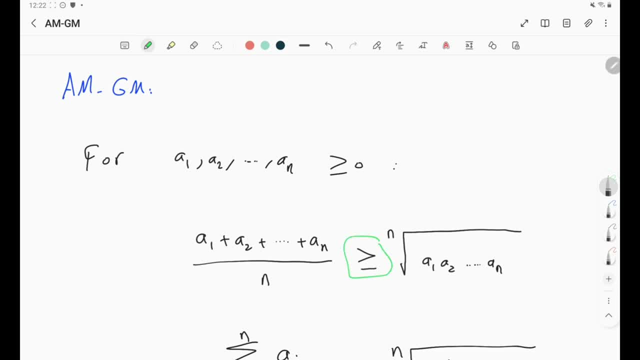 you have some equality case. Remember, we're just putting here greater than or equal to, So you really need to know when does equality hold? So in the amgm it's really simple: when all the numbers are equal, So we can just write here: